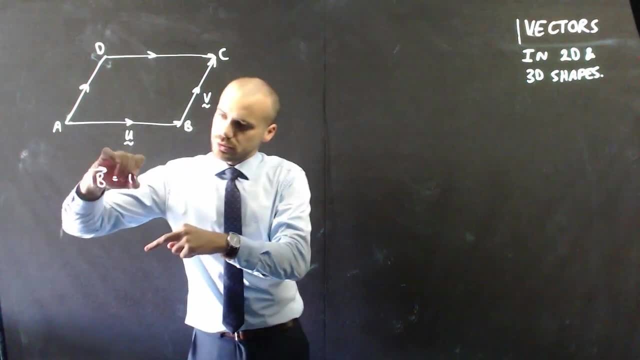 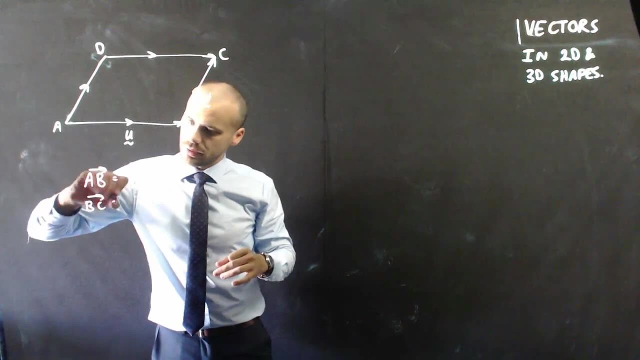 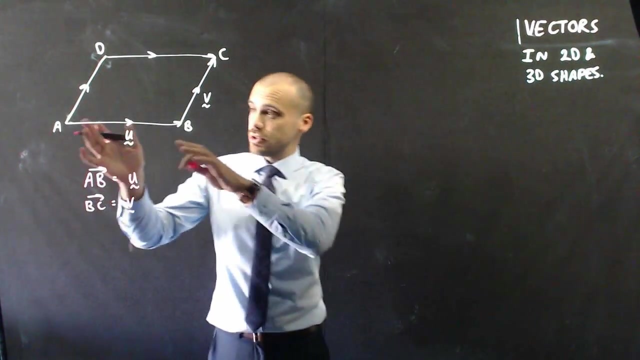 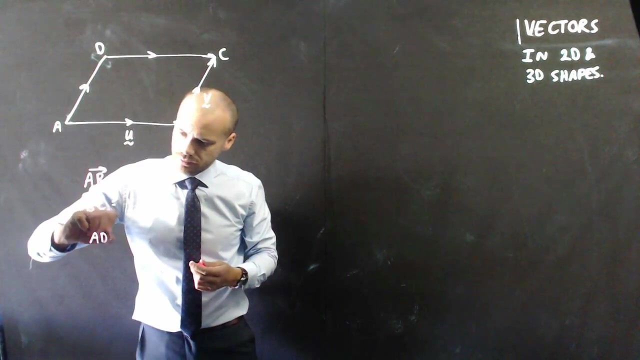 is equal to, and I've just called that vector U, And you can also see that the vector from B to C, I've called that V. Now, there is a bunch of other stuff that we can now define based on those two things. So, for instance, if I was to say to you what is the vector AD? So question mark, what is? 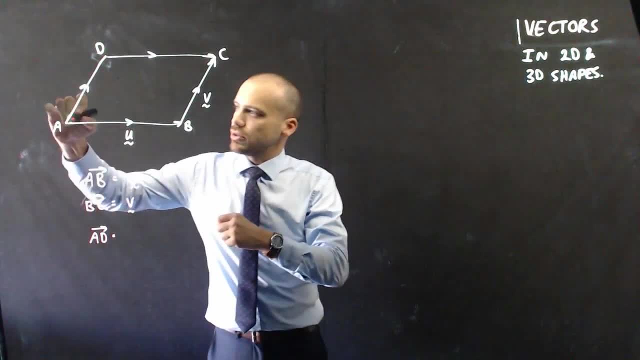 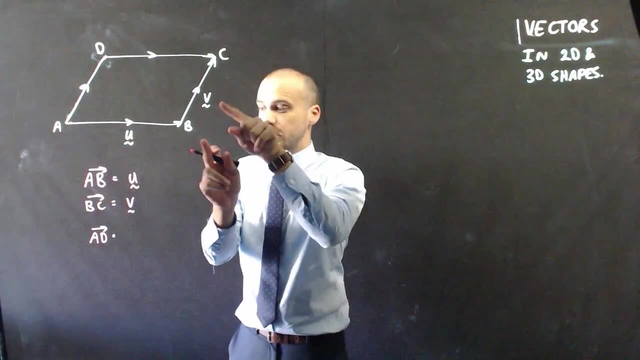 the vector AD. Well, the vector AD, so the line from there to there has the same direction and the same direction as the vector AD. So if I were to say to you what is the vector AD? Well, the vector AD has a magnitude as vector V, So actually that is the same as that, Even though 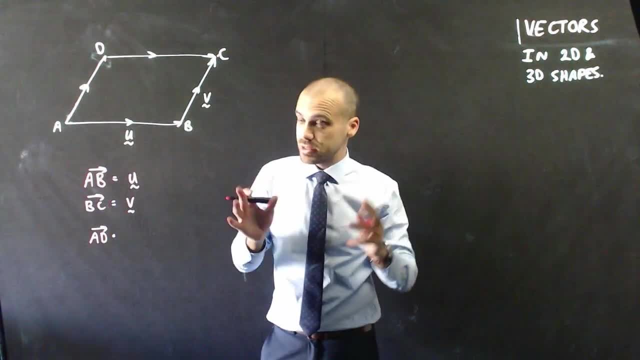 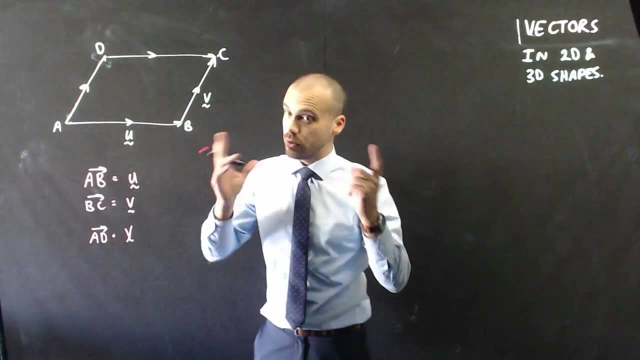 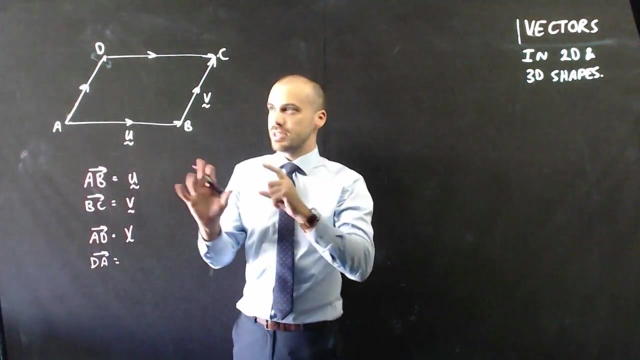 they're in different places because, remember vectors, they don't care what place they're in, we just need the direction and the magnitude. So we can say that AD is V. Now what about D to A? All right, so looking at D to A, that's a vector that's moving from here to here. 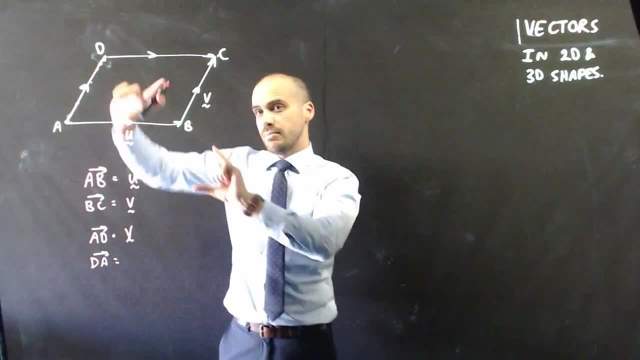 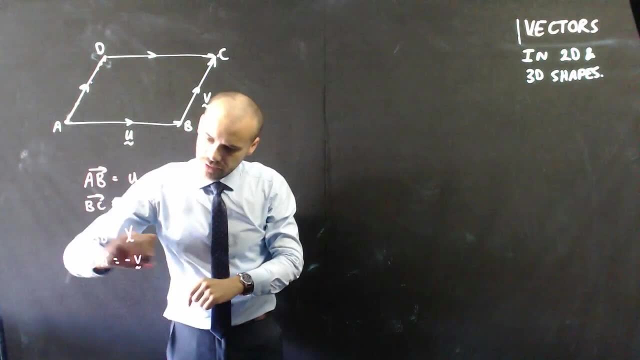 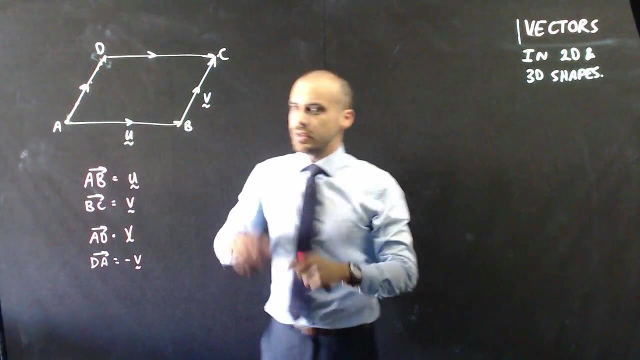 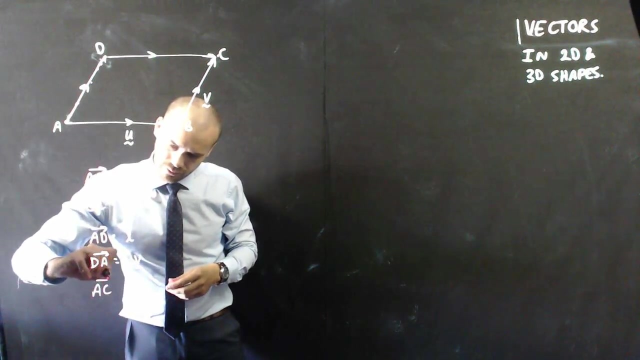 It has the same magnitude as V, but it has an opposite direction, So we can say that D to A is negative V, And we could do the same with U, by talking about CD or DC. Okay. now, the other thing that I want to look at in this is looking at the vector. well, what's AC? Okay, so let's look at AC. 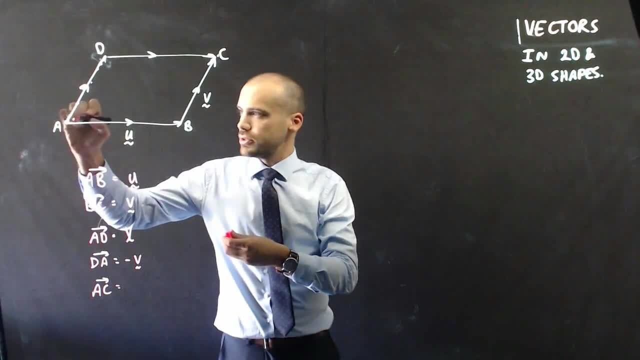 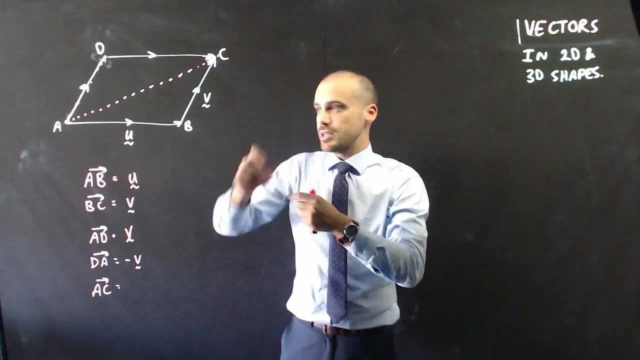 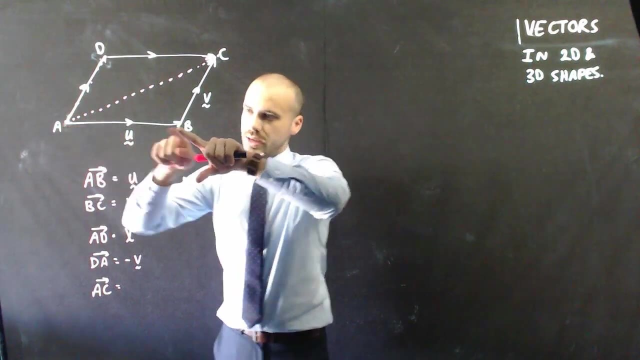 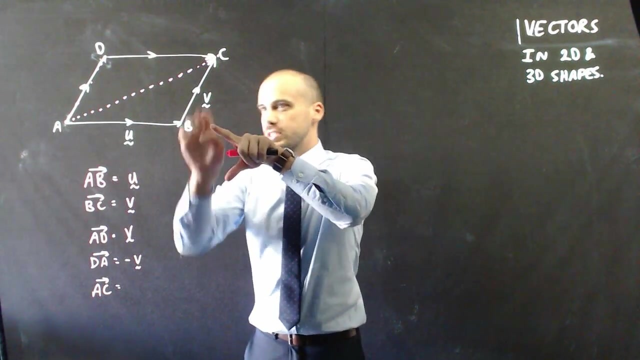 It starts from here And it goes all the way through there. Well, A to C starts at the tail of U and then joins the tail of V to the head of U, So it's actually U plus V, If you were to walk. 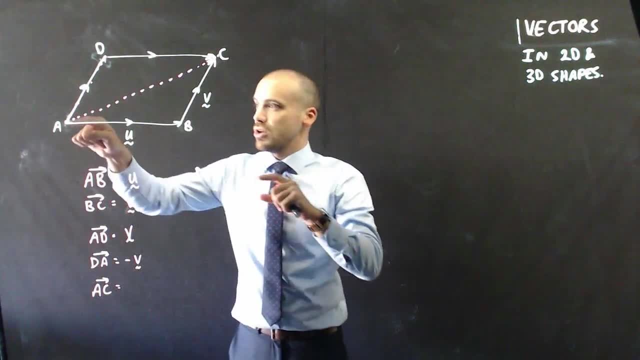 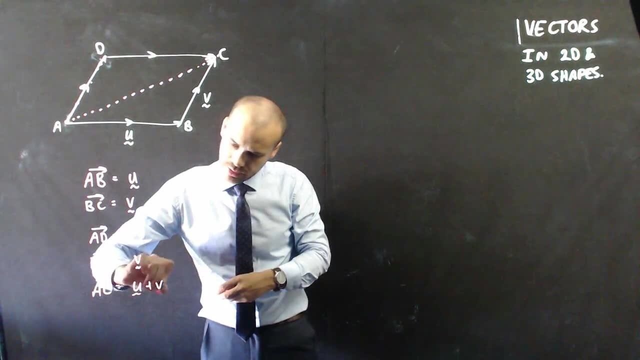 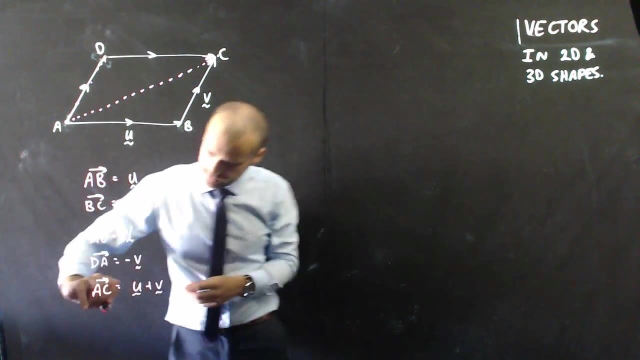 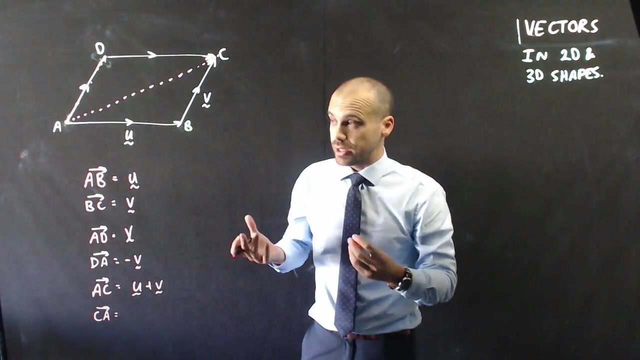 along U and walk along V. it would be the same as walking from A to C. So we can say that the vector A to C is equal to U plus V. Now what about the vector C to A? How could I walk from C to A? Well, obviously, I've got to do this whole thing in reverse. 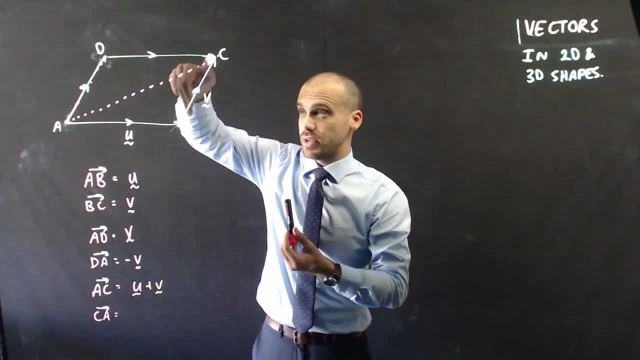 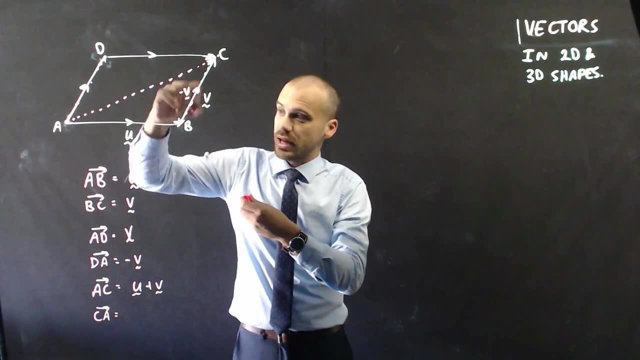 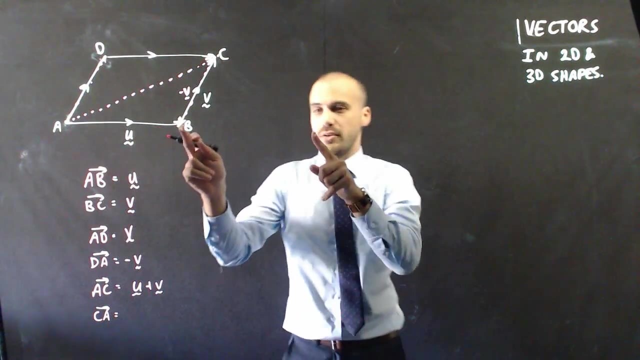 So if I were to take V and flip it upside down, I'd have negative V. That's negative V in that if it's going in that direction, And if I were to take U now and add it to that? well, if I were to take U and add it to that, I'd end up over here, because that's U in. 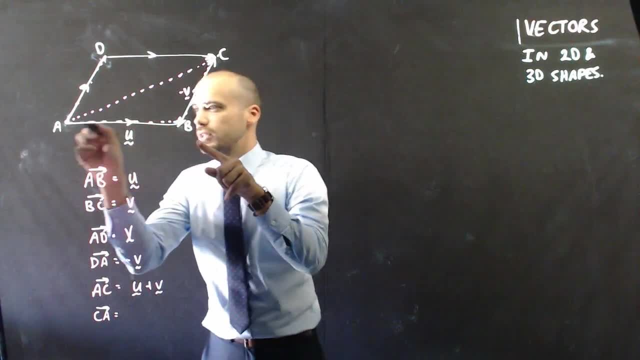 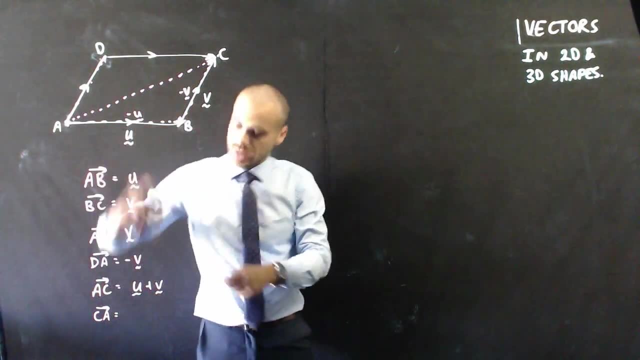 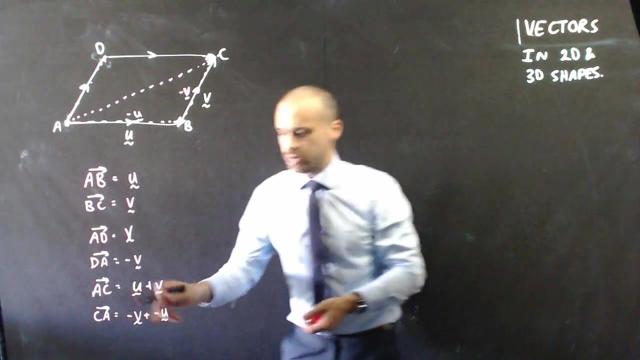 that direction. But if I were to take negative U moving in the other direction, now I'm in business, So I can say that C to A is negative V plus negative U, Or just get rid of that plus and say it's negative V, negative U. 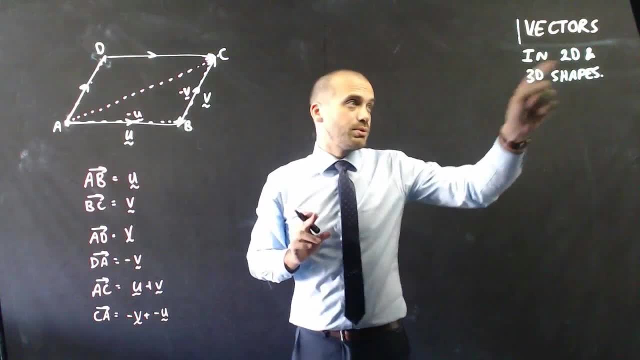 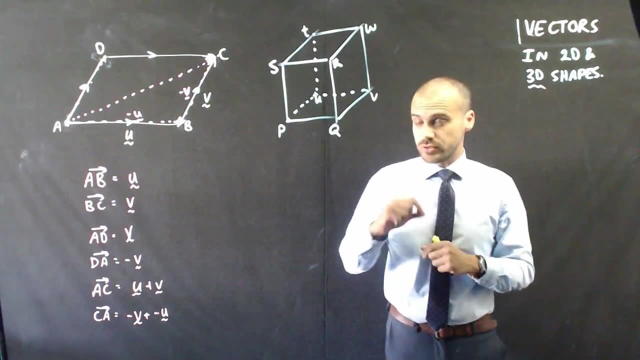 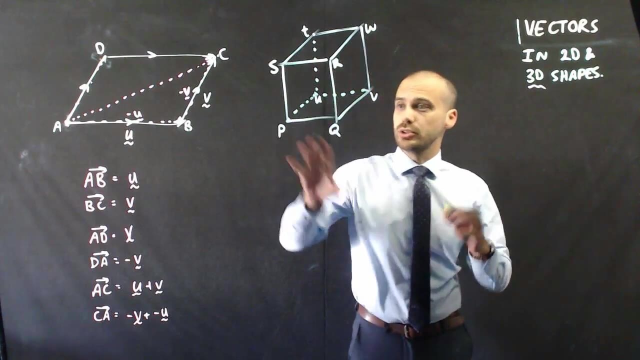 All right, so there's a parallelogram, But I said we were going to do 2D and 3D shapes, So vectors don't only have to exist in two dimensions. Three dimensions is where we'll use vectors a lot. Here's a cube: P, Q, R, S, T, U, V W. Now if we were to find the vector? 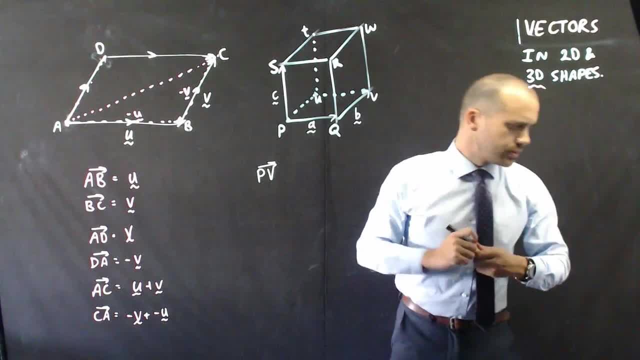 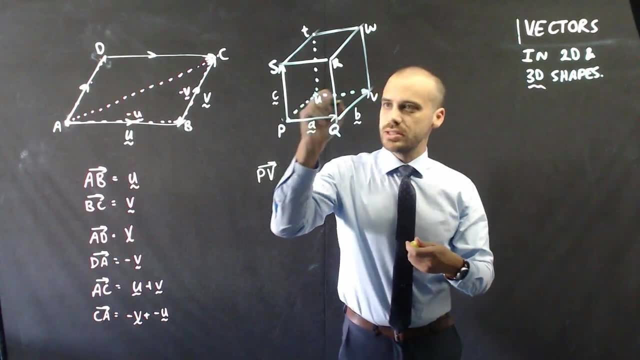 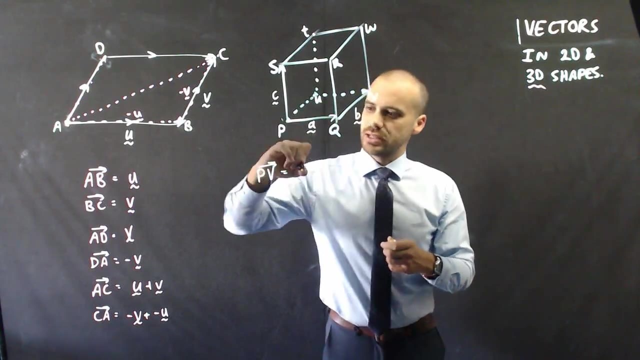 P V. oops, I forgot to draw my vectors in. so that's vector a, that's vector b and that's vector c up here. so the vector from p to v across the bottom of this cube or rectangle, rectangular prism maybe, is vector a plus vector b. now we can. 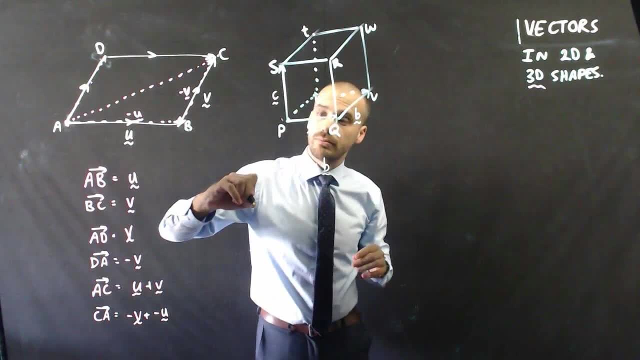 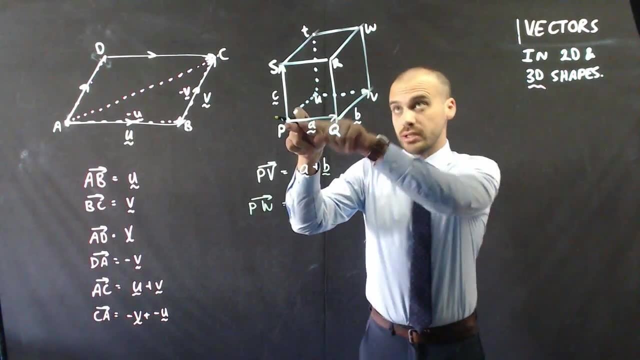 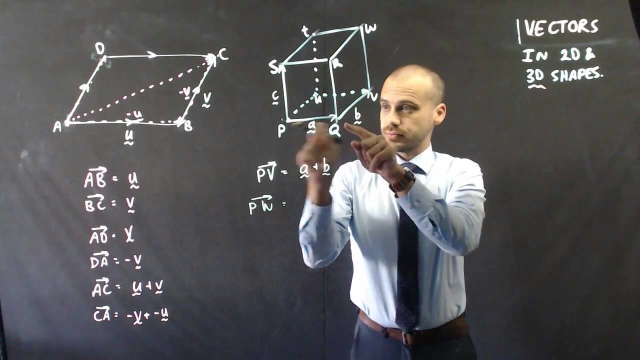 start moving into that three-dimensional stuff and saying, well, what about from p to w, from this front corner to this back corner, here, right through the middle of the rectangular prism? well, if we take a, if we, if we were to travel along a and then travel along b and then travel. 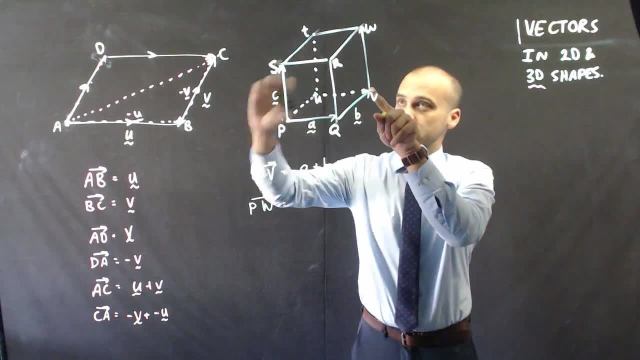 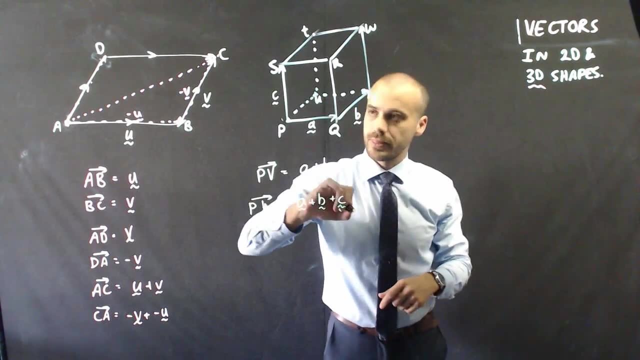 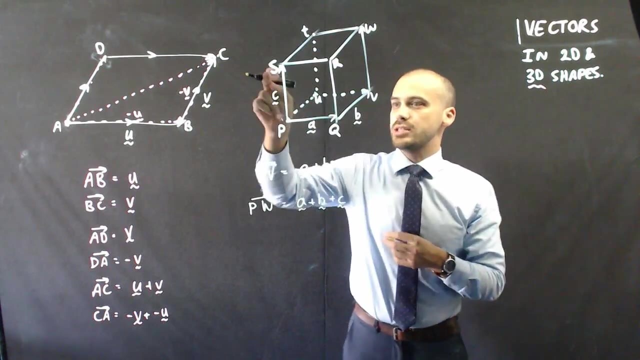 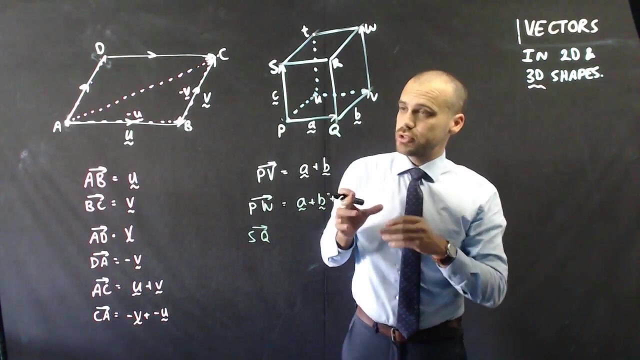 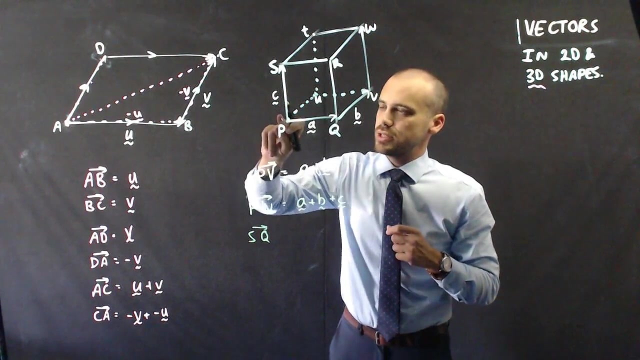 along c because remember, that's c, so that's also c. it's just going to be a plus b plus c. okay, so now what if i were to go s to q? so to travel from s to q i would have to travel the backwards of c. all right, so negative c.